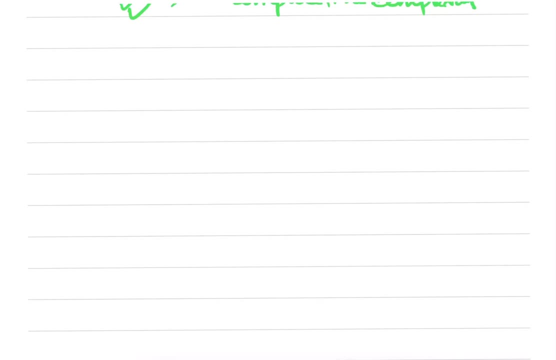 Hi everyone, welcome back to our channel. Let's start with the Naive algorithm. First we will see the concept, then we will see the designing part of algorithm and we will analyze the time complexity. So the concept says we will be having a text and a pattern. 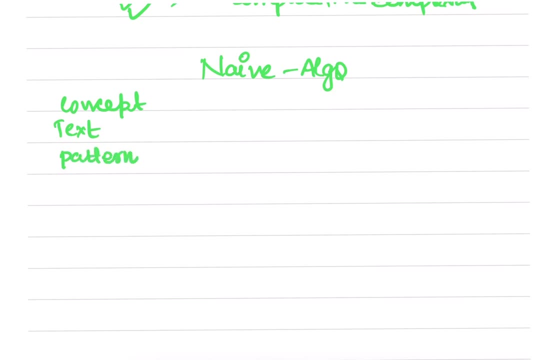 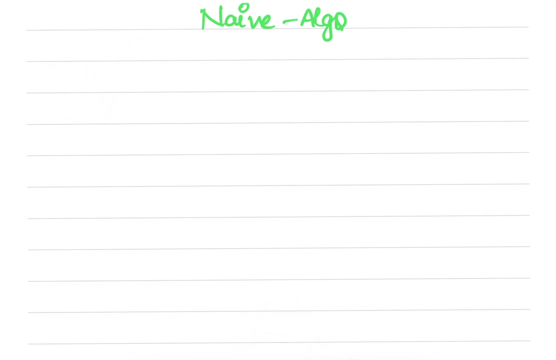 So you have to start comparing the pattern from initial character of the text And if any character of pattern doesn't matches, you have to ship to the consecutive character. That is, for example- let's take an example. For example, let text be A, B, C. 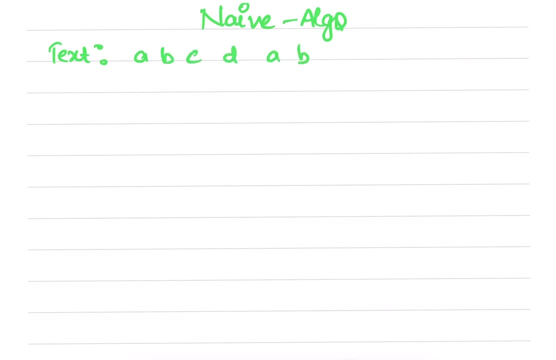 A B, C, D, A, B, F, A, B, E and G, And let's say a pattern is A B E. So you need to find A B E in this text, right? 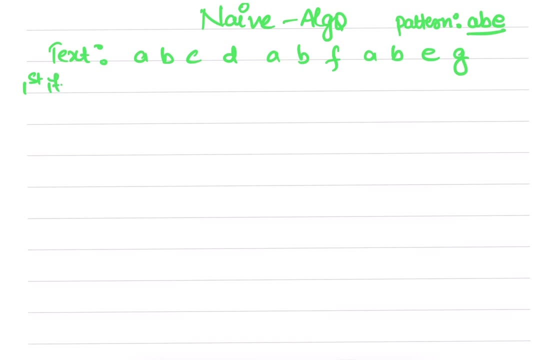 So let's start with first iteration. I will start from the initial character of the text. So A, B, E. A matches with A, yes, B matches with B, yes, But C doesn't matches with E. So how many comparisons are made? 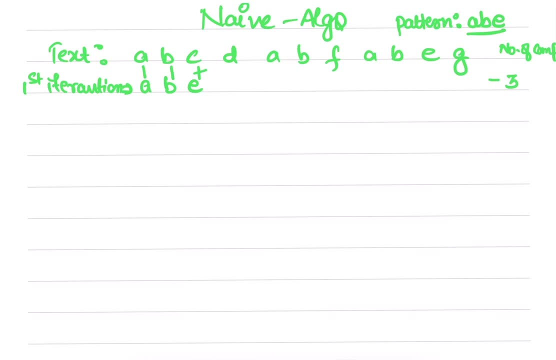 So I will just write number of comparisons. So number of comparisons made are 3.. So now I will ship to its consecutive letter of inner text. So A, B, E. Now I will ship here. Now, if you see, here B doesn't matches with A. 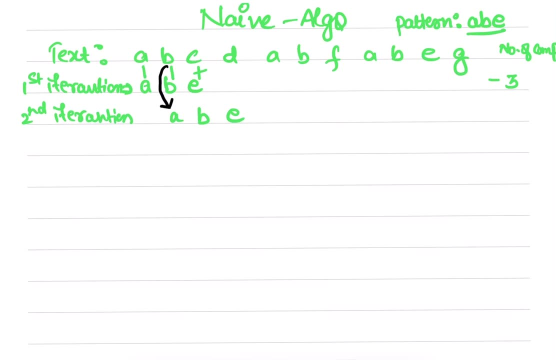 I will compare again. and B doesn't matches with A, So I will stop here. only So number of comparisons made are 1.. Then I will ship to its consecutive letter of inner text, Third iteration: A, B and E. So can you see here. 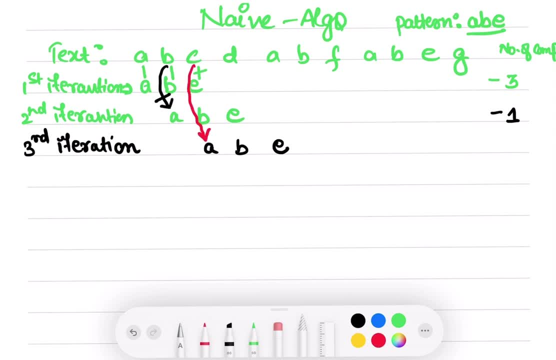 This C doesn't matches with A Right, So only one comparison is made. We will go to fourth iteration, So I will just ship to its consecutive text. So it will be A, B and E. So if I see this D doesn't matches with A. 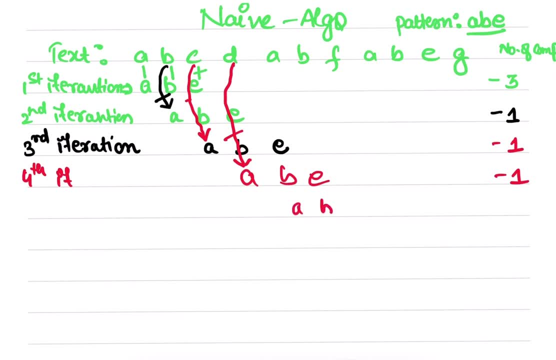 So only one comparison and I will ship it to here: A, B and E. Let me write it. Fifth iteration: Here you will see that A matches with A- Yes. We will go further: B matches with B- Yes. 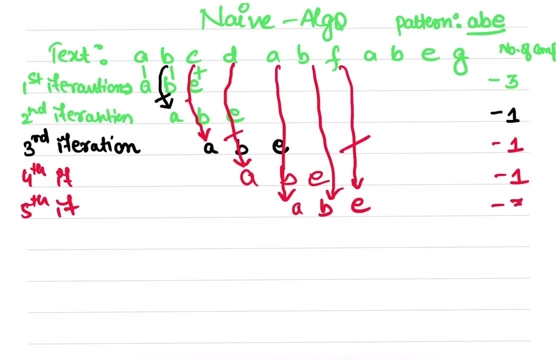 But F doesn't matches with E. So three comparisons are made, But we didn't get the text. So sixth iteration: A, B, E. Again, I will ship it Now. you will see that this B doesn't matches with the A. 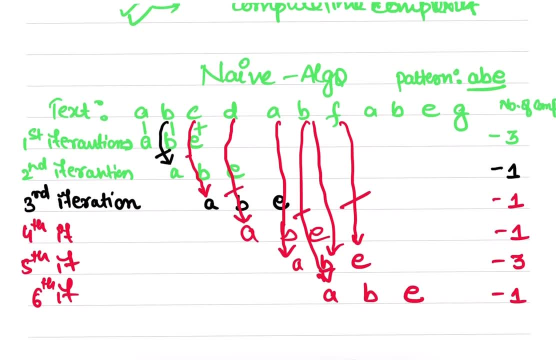 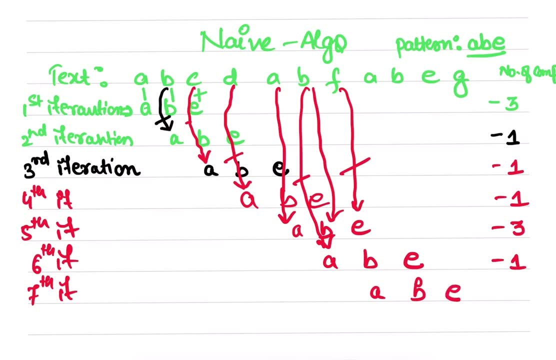 So only one comparison is made. And the seventh iteration. if you see, Let's ship A, B, E. So let me change the color So you will see this F doesn't matches with the A, Hence one comparison. Let's go to eighth iteration. 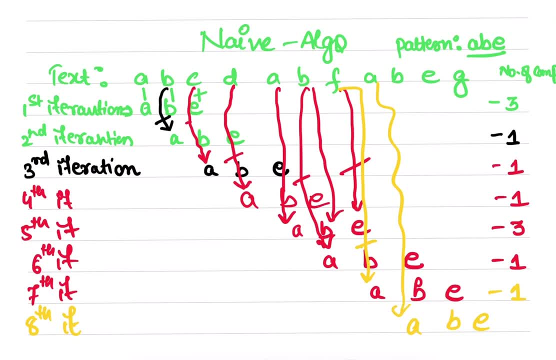 A, B and E. You will see this A matches with this, This B matches here And this E also matches here. So all three characters of pattern matches with the text. Therefore, we found, And hence we have made, three comparisons. 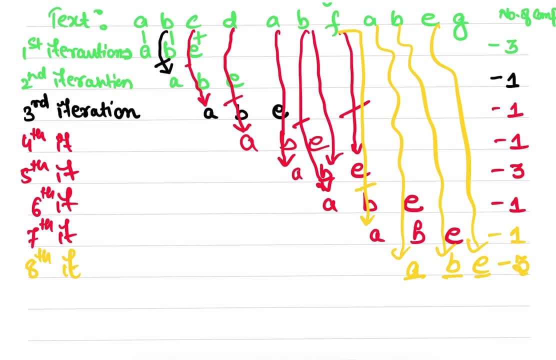 So, therefore, we got the pattern in our text. So therefore, the conclusion of the algorithm is that we went till eighth iterations. We got the pattern in eight iterations. And what are the number of comparison meets? The number of comparison meets are 3 plus 3, 6 plus 9, 10,, 11,, 12,, 13,, 14.. 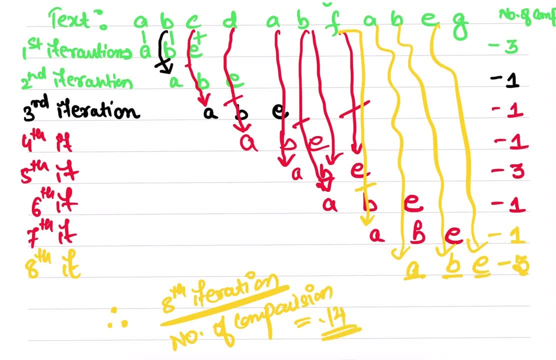 14 comparisons. So this is how Naive's algorithm works. Now let's design the algorithm for this. So, as you can see here, What we have done is We have text, We have pattern, Right, So let's design the algorithm. 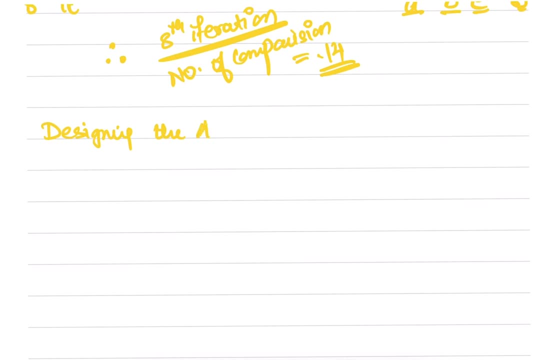 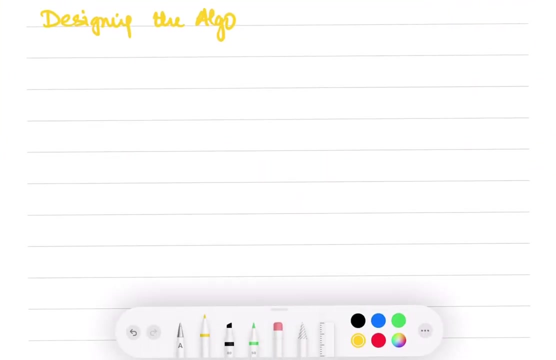 Designing the algorithm? Right, Let me change the color. So what will be our input? Input will be our text And the pattern, Right. And what will be the output? Your pattern found or not, Right? So let's say I write Naive string algorithm. 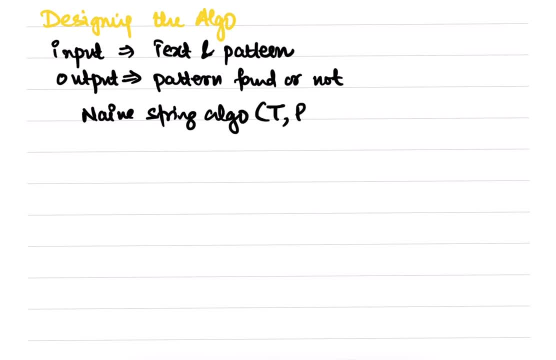 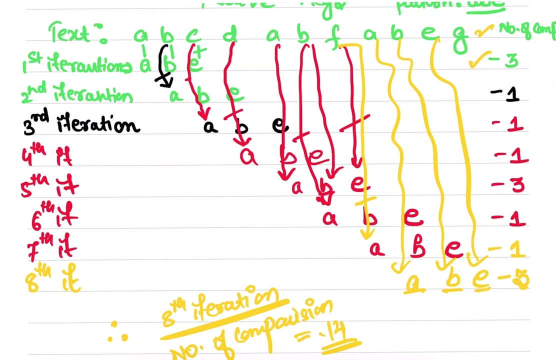 Algorithm. So what will be input? Your text and the pattern. So you will be giving, let's say, n, That is your text length will be a pattern length. so what you are doing here is you're comparing it right. you're comparing pattern with the text and if any of doesn't matches, you're. 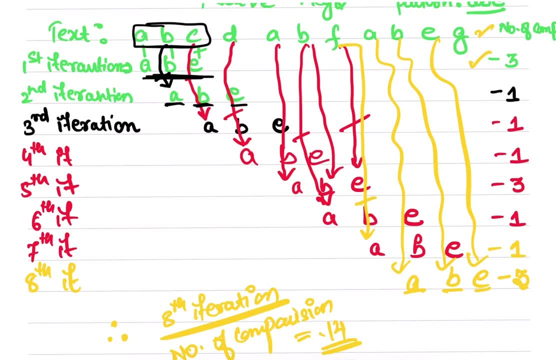 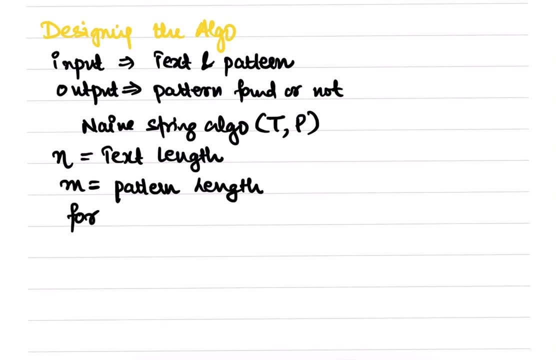 again, in comparing all the alphabets, all the alphabets of the pattern, with the consecutive, that is, there will be a for loop. for, let's say, s equals to zero to n minus 1. now it's your choice whether to take s equals 0 to n minus 1 or. 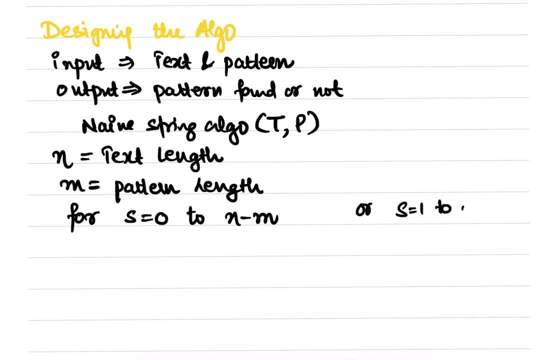 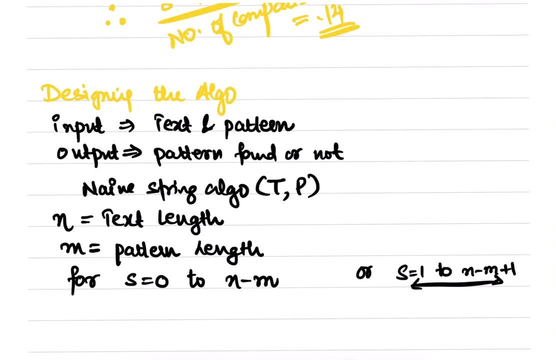 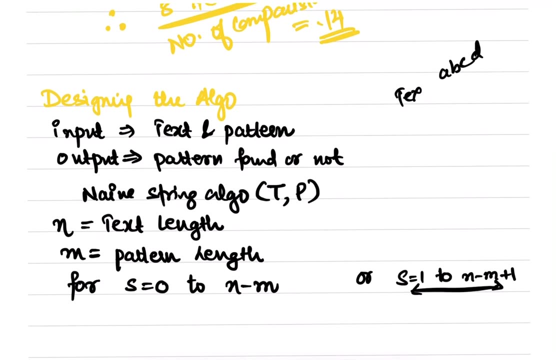 you can go like this: s equals to 1 to n minus m plus 1, your choice. because, for example, let's say your text be ABCD, right, and my pattern be, let's say, xy. so how many characters? four, what is xy? two, two characters in a pattern. 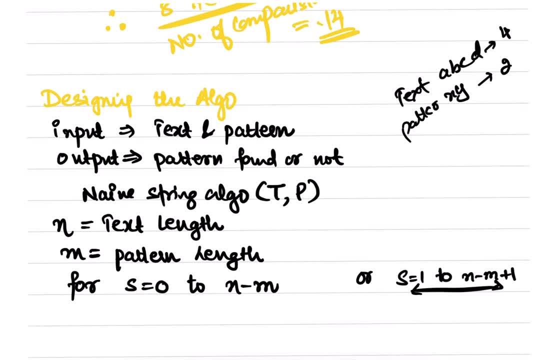 and four characters in a text, right. so now how many comparisons i'll make. let's see: x- y is here, first loop, then x y, second loop, right, then x y, third loop, right, that is three times loop should work. so what is n minus m? four minus two, that is from zero to. 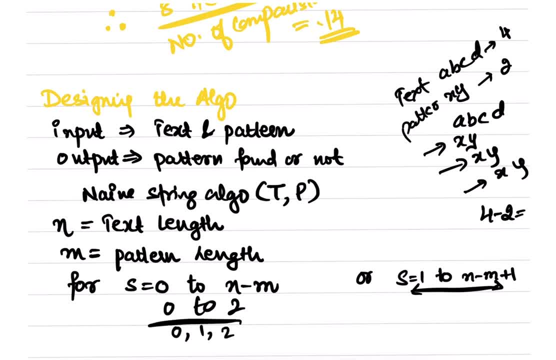 two, that is zero, one and two. so loop is working three times: first loop, second loop and third right. or if you says from one, so here it will be n minus one, that is four. minus two is two, plus one, that is three. so should loop one, two and three. are they getting? 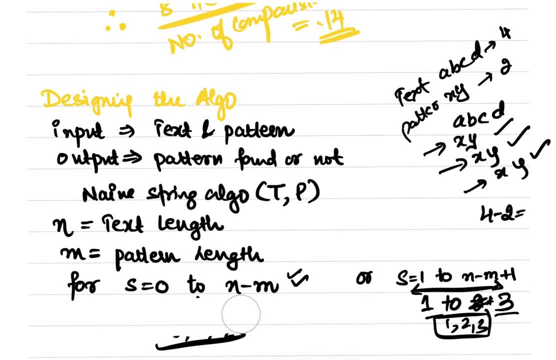 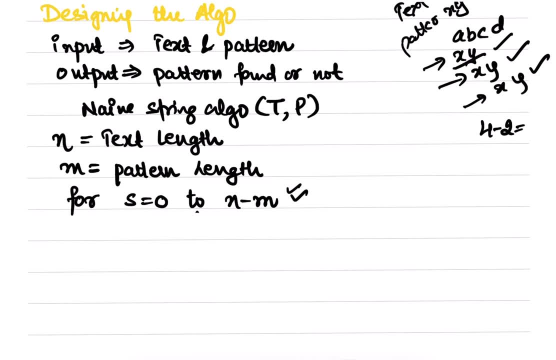 right, this for loop, right? i hope it's clear to you now. let's move further now. so this loop is clear right now. what do you do in particular iteration? you just compare if the pattern, whatever the pattern you have- matches with the text. right, if it matches, just print. 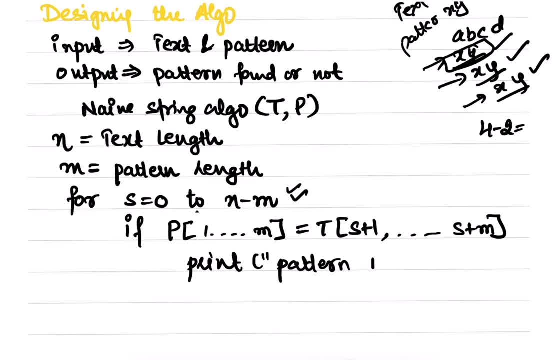 pattern, whatever the p or column at shift s right, right. so this is your algorithm. so it's a very easy algorithm. naive bias, basically use brute force. actually, that's why it becomes very easy. you just need to shift to its consecutive text pattern. or you can say: 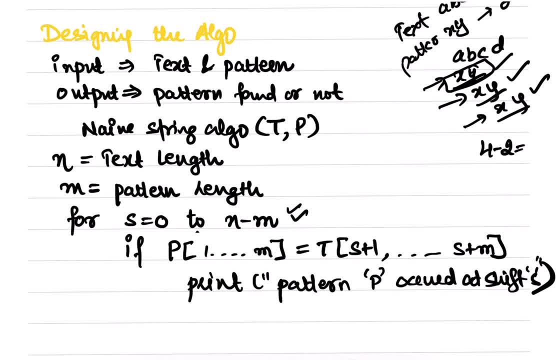 corrector, sorry. so designing the algorithm now, if we have to analyze it, if we need to analyze this part, so can you see, this loop works till n minus m plus one right, n minus m plus one. i already told you why this: because i have taken zero. so if i have taken one, two n minus m plus one. 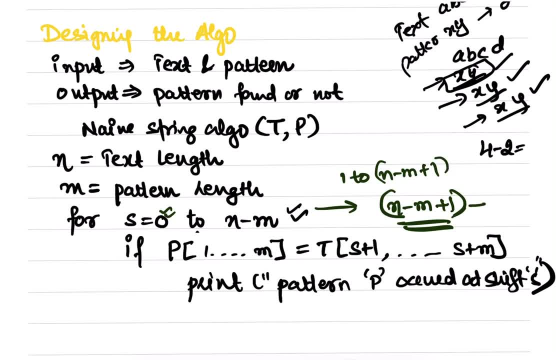 then i think it will be very much clear that this for loop works for n minus m plus one. so i i showed you right. so if that's what i wanted to be, so first take it to enter ingredients. so this loop works for n minus m plus one time. and in worst case, what kind of possibility that we have to compare all the 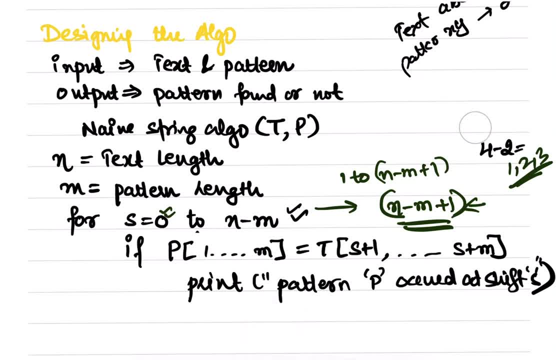 connectors. so here, if you see in this example only abcd, example a-, b-, c- d, if you see xy, i have to compare x also, y also, x also, y also, also y also. so I have to compare M in worst case. so therefore, therefore time: 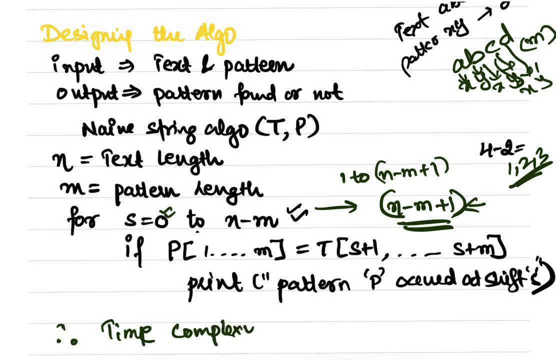 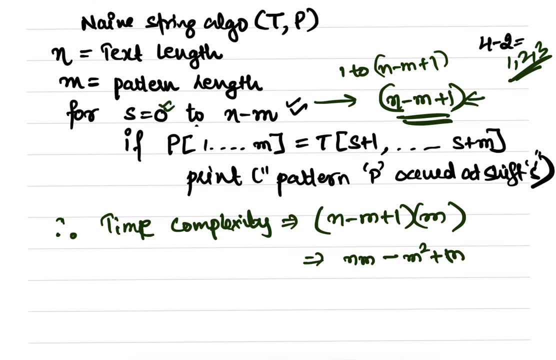 complexity, time complexity is nothing but N minus M plus 1 times M. so if you solve this equation, you get N, M minus M, square plus 1 or plus M, and in my basics of string matching algorithm video I already told you that, according to the analysis, N is always greater than M. therefore we neglect M. square equals to: 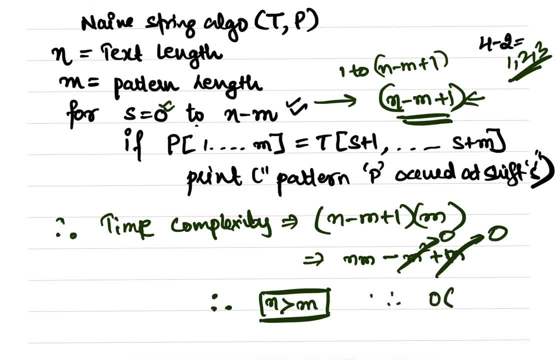 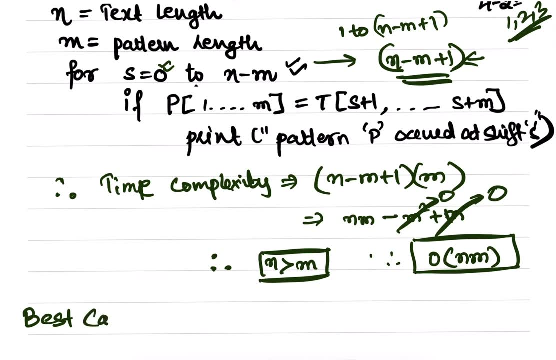 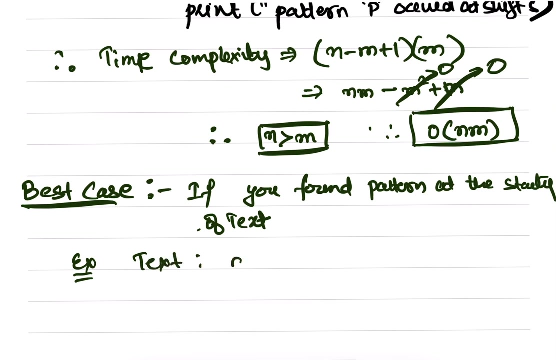 0. we neglect this. therefore, the time complexity is M. therefore, time complexity is M. now, what is the best case? what is the best case for this? best analysis? best case now, best case is if you found pattern at the starting of the text, right starting of the text. for example, let's say, your text be ABC, A, B, A, B, C, D, right and your 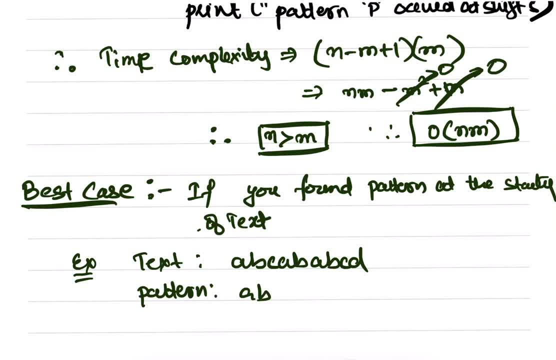 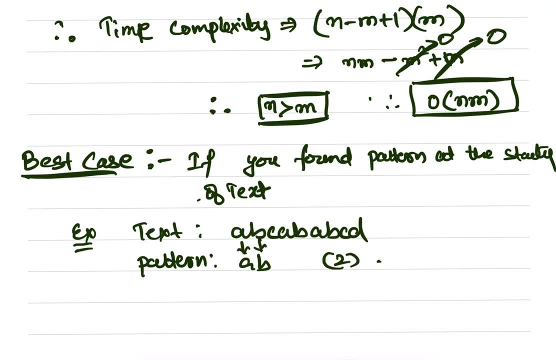 pattern is this: AB. so in the first attempt, only that is what you will do. A and B. only two comparison, that is, M comparisons only. so therefore, time complexity for best case is O of M. you just need to do M comparison right. so only two comparison. you have to do that. 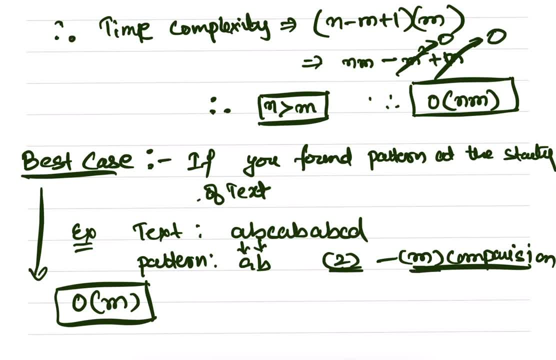 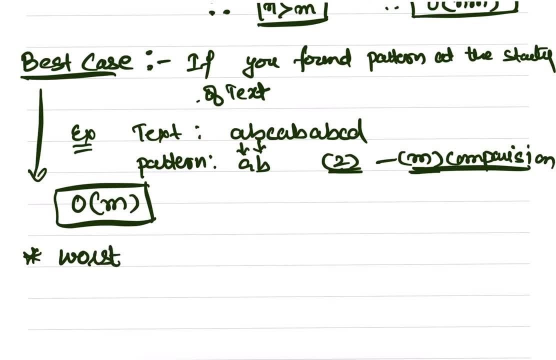 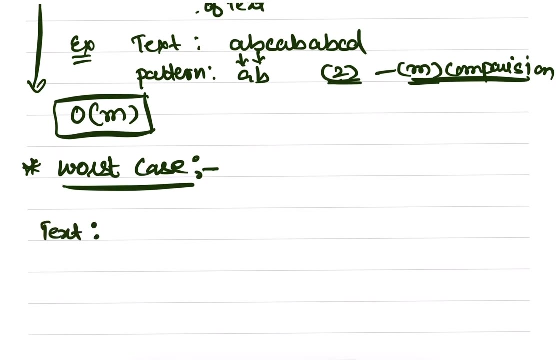 is M comparisons and you will get your pattern in a text. now, what's the worst case? that's very tricky here. if you say worst case is the thing that if we found a pattern at the end of the text, let's analyze that thing, great. so let my text be A, B, C, D, E, F, G and H and. 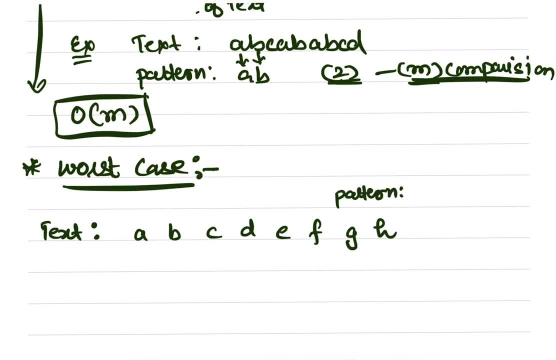 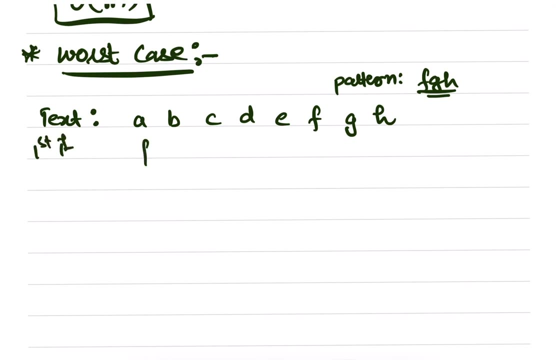 let's say my pattern be F G H, right, so it's. this pattern is here right at the end of the text, so I think it will be a worst case, right? let's see, let's analyze it. so your first iteration goes like this: I think F G H. so it doesn't matches. only let me write number of comparison here. 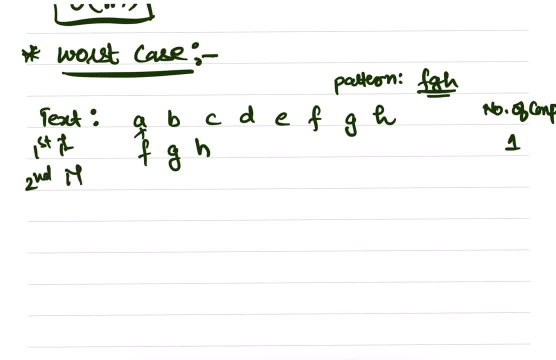 so it's one. second iteration: F G, H, B doesn't matches it. F, one comparison and move further. third iteration: F G H. see it doesn't matches with this. I again I'll move forward. fourth iteration: F G, H, D doesn't matches with F and move. 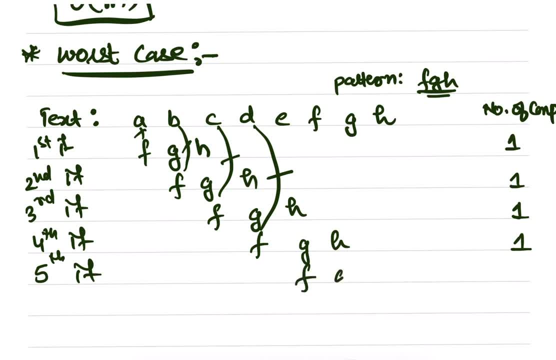 further fifth iteration: F, G, H, E doesn't, matches with F, one comparison. and move to the sixth iteration, F, G, H, F matches with G or, sorry, F matches with F, G matches with G and H matches with H. three comparison, so two. total number of comparisons are 1,, 2,, 3,, 4,, 5 and 8.. So, therefore, total number of 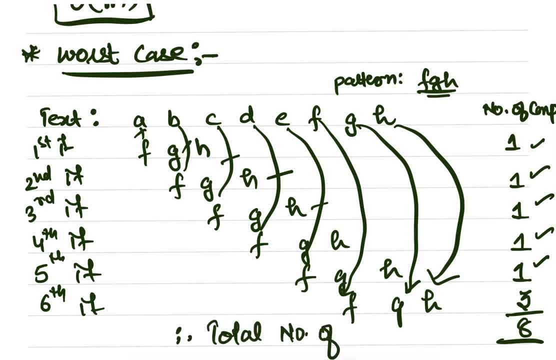 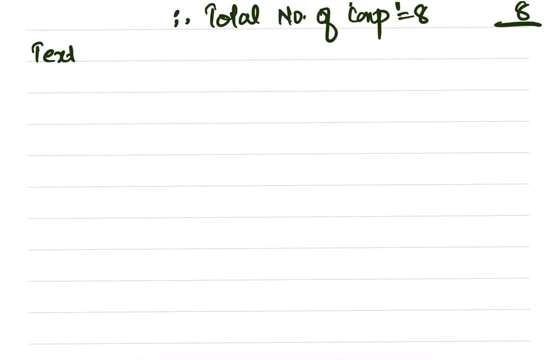 comparisons are 8.. So do you think this is a worst case? Actually, this is not a worst case. Now why? Let's take one more example, then it will be very much clear to you. So let's practice one more example: A, A, A, A, A, A, A B. Let's do this So. 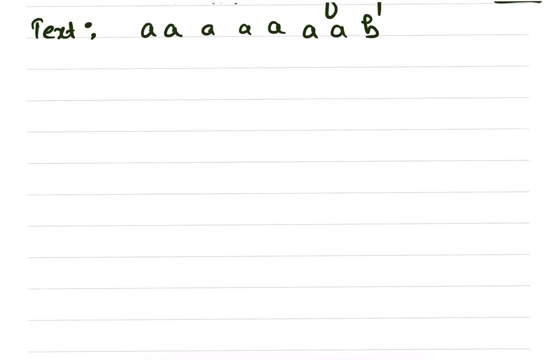 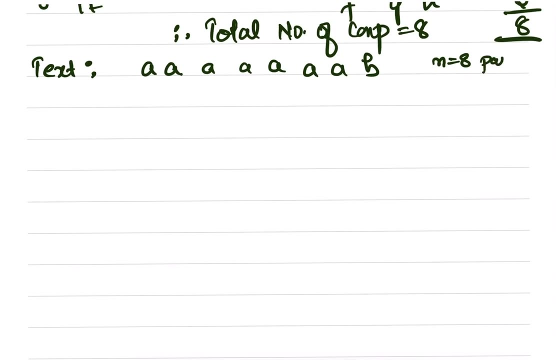 1,, 2,, 3,, 4,, 5,, 6,, 7,, 8.. So what's the value of n here? It's 8.. And let's say pattern B: A, A, B, Right? So let's first, let's start with the first iteration. 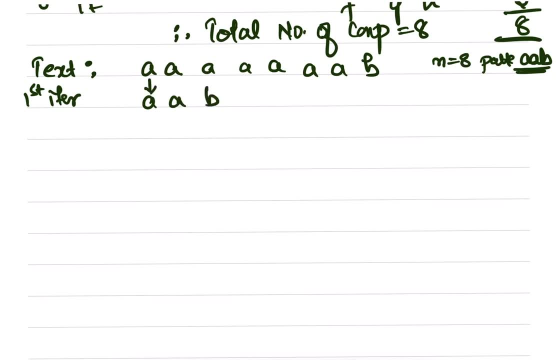 here: A, A, B, So this matches this matches this doesn't match. So number of comparisons 3. Second iteration: A, A, B, This matches, this matches. this doesn't matches Three: 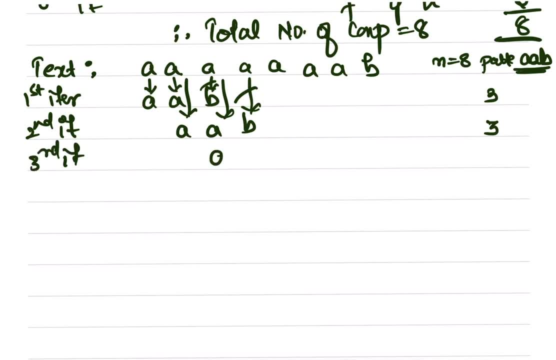 comparisons: Third iteration A A B: This matches this: matches this doesn't matches. Three comparisons again. Fourth iteration A A B. This the matches this, matches this, doesn't matches three comparisons again. fifth iteration a a B. I think I'm going right, right, so this matches this, matches this: 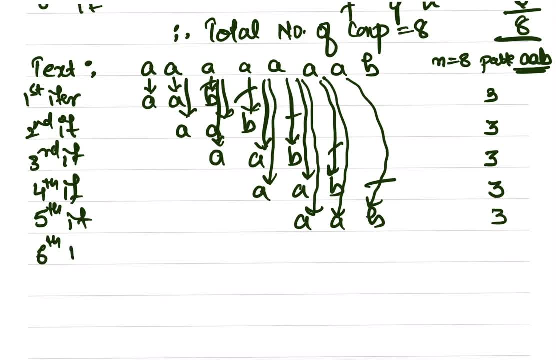 doesn't matches. third iteration: go to six iteration a, a, B. here, if you see, this matches, this matches this also matches. so three comparison. so number of comparison here: number of comparison: how many? 1, 2, 3, 4, 5, 6, that is, 3, 6, 18, 18. 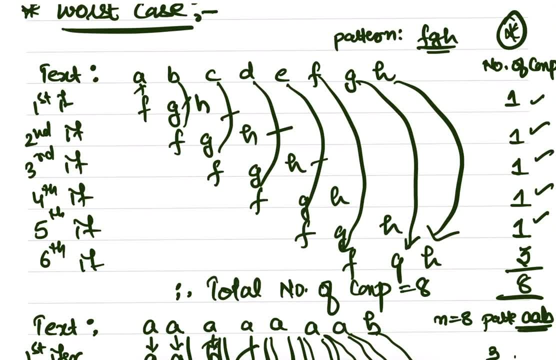 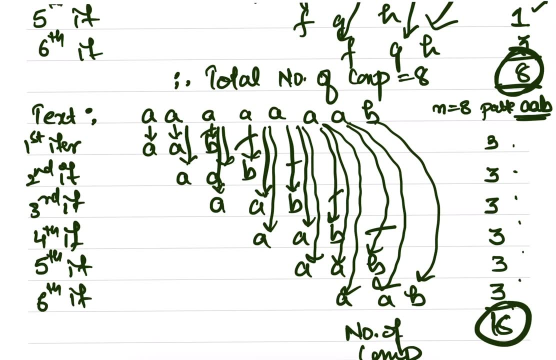 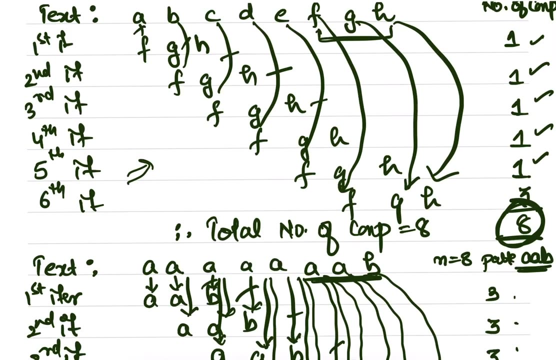 comparisons. now, here you will see: you just got eight comparisons when your text was, or your pattern was, at the end of the text. here also, you got 18 comparisons. sorry, 18 comparison when your pattern was at the end of the text, but the difference between this example and this example is that here, at each iteration, 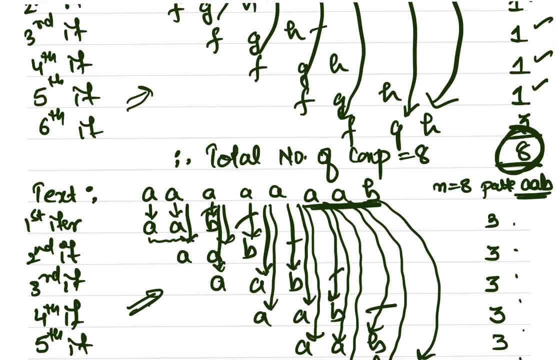 we were comparing all three characters of the pattern, that is, at each iterations we were comparing all M characters of a pattern. so whenever, so whenever, we were comparing all M characters of a pattern, so whenever. so the condition comes in which pattern is present at the end of the text and you 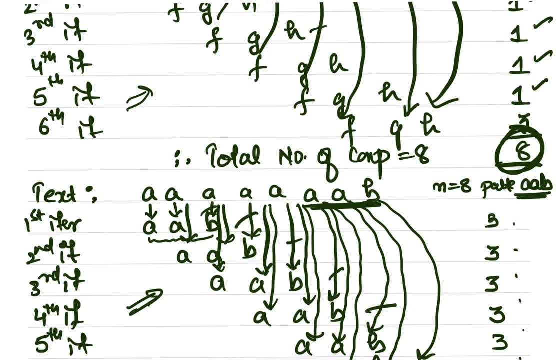 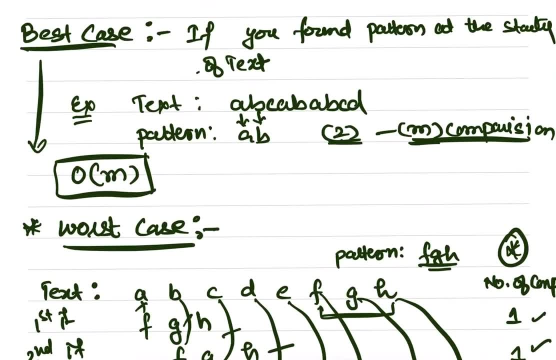 the condition comes in which pattern is present at the end of the text and you are comparing all characters of the pattern in each iteration, that is, are comparing all characters of the pattern in each iteration, that is considered as a worst case. so, in addition to worst case, if pattern is, 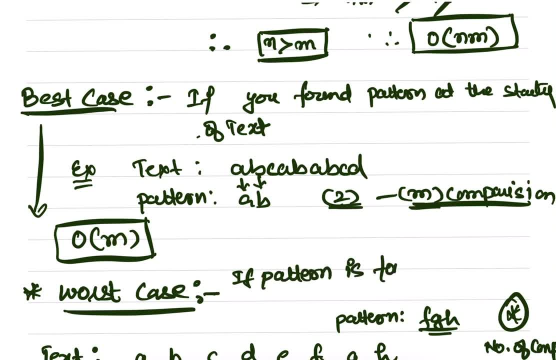 considered as a worst case. so what's the found? is found at the end of text carats. at each operation it should make a make a five times will be considered as a worst. so what's the time complexity for all parts reading. and this is the following: